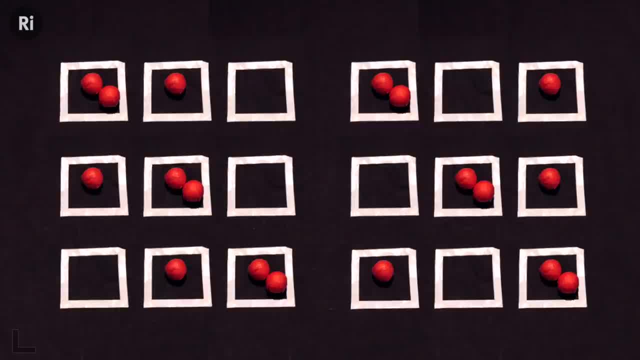 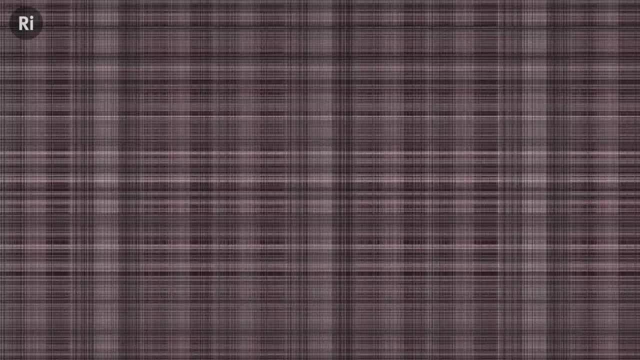 spread out to a different degree. That's straightforward enough, but when you scale it up, even by a factor of ten, things get much more complicated. Counting the permutations becomes impossible. Now, if you imagine that there were trillions upon trillions of atoms and 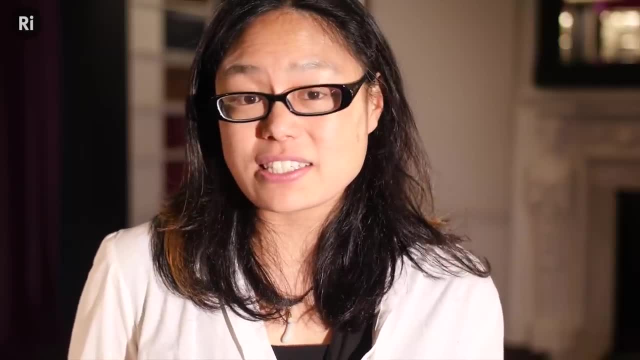 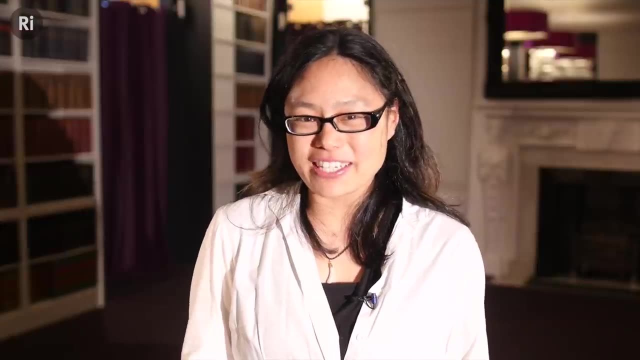 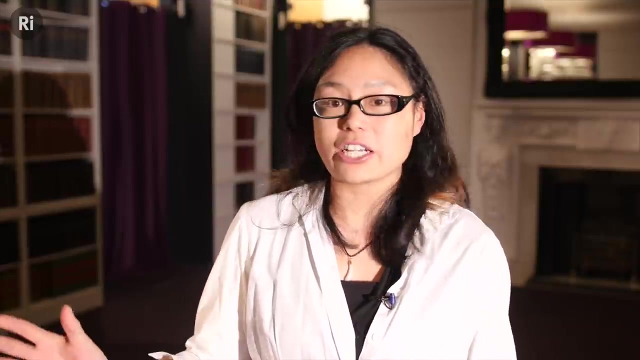 trillions upon trillions of boxes, then statistically you could see that it's much more likely that the atoms would be disordered rather than ordered. Perhaps the most significant conclusion from the second law of thermodynamics is the concept of the arrow of time, which tells you which direction time is traveling in. 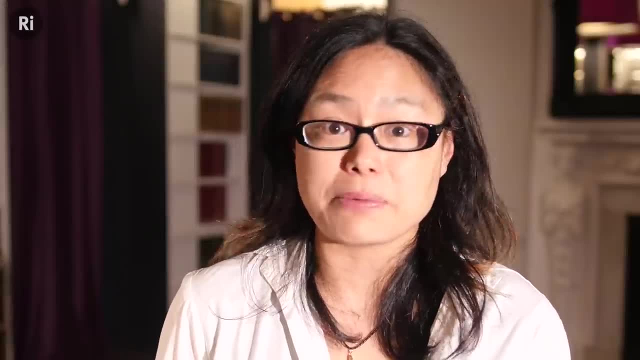 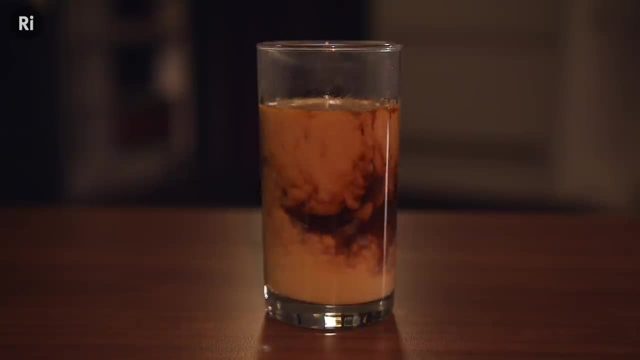 For example, if a process generates entropy, it will happen spontaneously and will be irreversible unless you input more energy. When I pour cream on my coffee, I wouldn't be surprised to see the two liquids mixing and becoming more disordered over time. I would, however, be 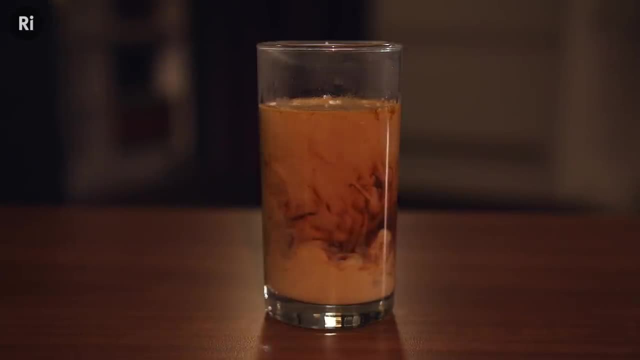 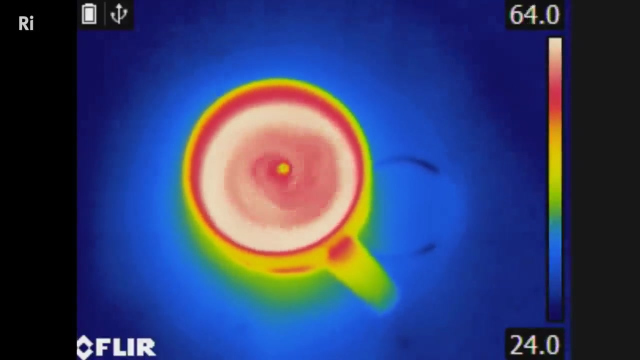 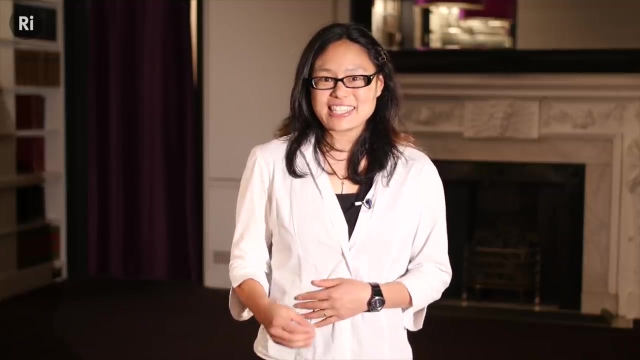 surprised if the cream and coffee separated again after I had stirred them. An ice cube in coffee will melt and become a more disordered liquid, but under those conditions it cannot spontaneously reform itself back into an ice cube. So you might be tempted to think that if this is true and if 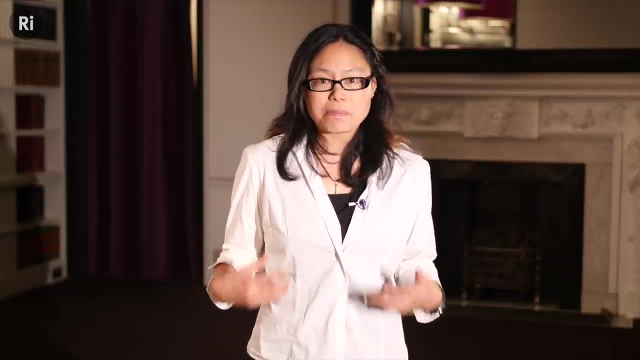 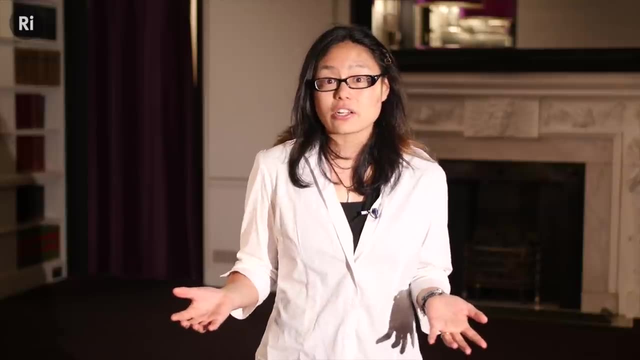 entropy can never be decreased, then it's just a matter of time before you can do anything about it. Then how can human beings or more complex living organisms even exist? Well, the key here is that humans are not a closed system, so we're always exchanging heat with our surroundings and we're decreasing local entropy at 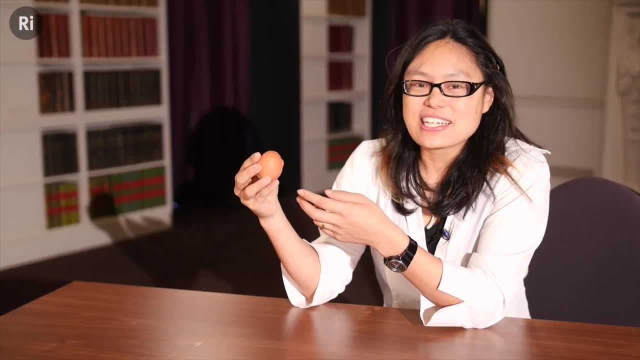 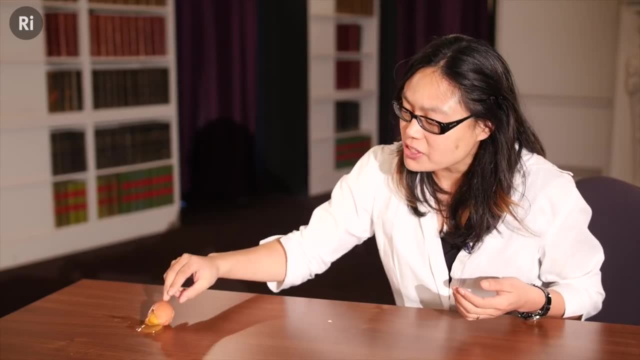 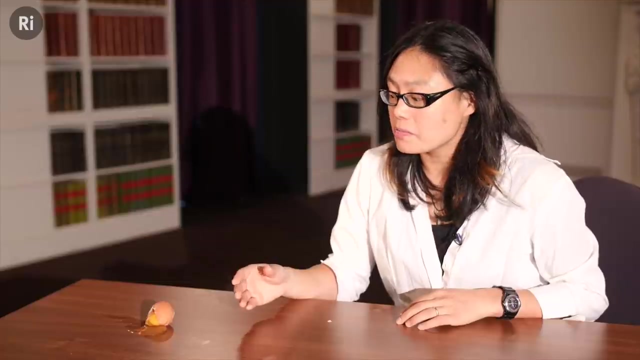 the expense of the entropy of our environments. So if I take an egg and I drop it, then the second law says that this egg will never spontaneously unbreak itself. But even the initial laying of the egg doesn't violate the second law, because the hen took a lot of food and broke it. 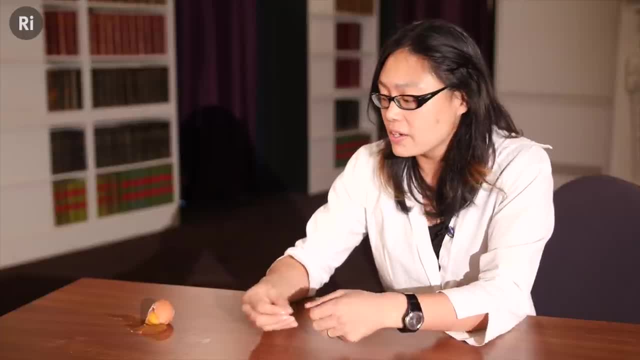 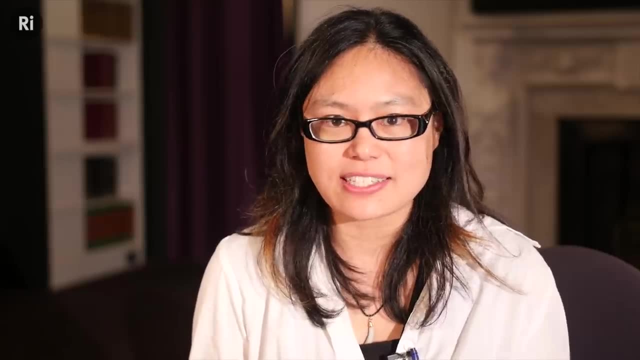 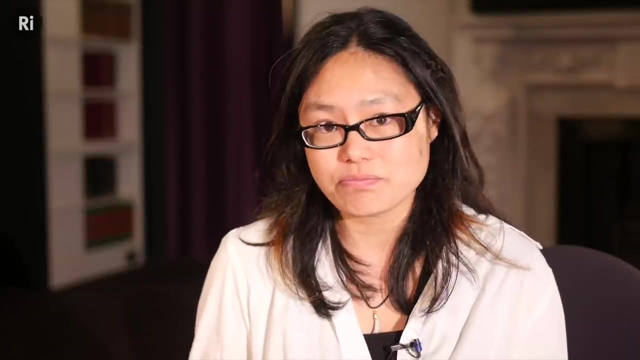 down, so creating a lot of molecular disorder or entropy in order to make this egg that I've just broken. So the second law states that a spontaneous process generates entropy and involves heat moving from a hotter body to a colder body. Now, a refrigerator doesn't violate the second law of thermodynamics. 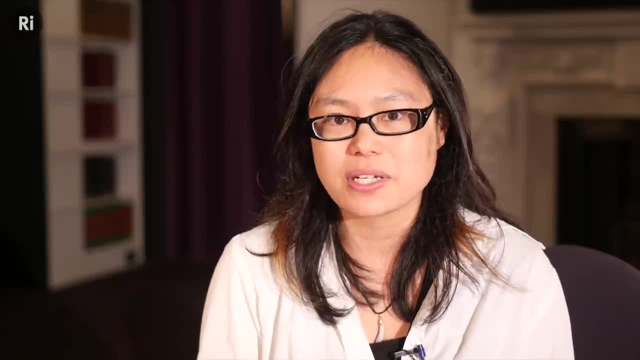 because it's not a closed, isolated system. Where a refrigerator is not a closed, isolated system, it's a closed system. Where a refrigerator is not a closed, isolated system, it's a closed system. So we're continually inputting energy in the form of electricity to try and keep.